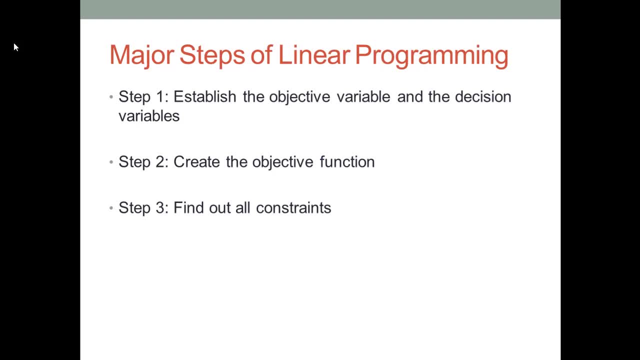 is facing the limited amount of resources. That's why we want to identify the constraints. Then we want to build the objective function according to the constraints, according to what we have in reality. This is the major step of performing linear programming. If you just get in touch with this topic, if you are not very familiar to the fundamentals of linear programming, 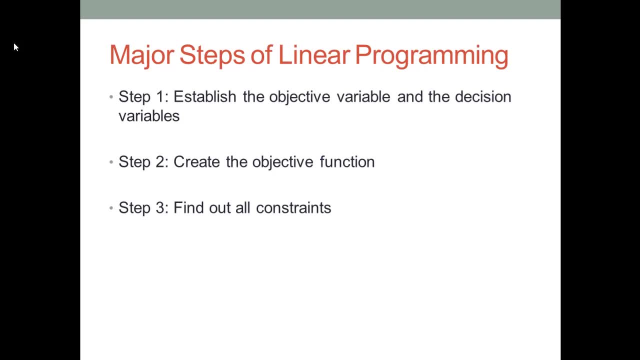 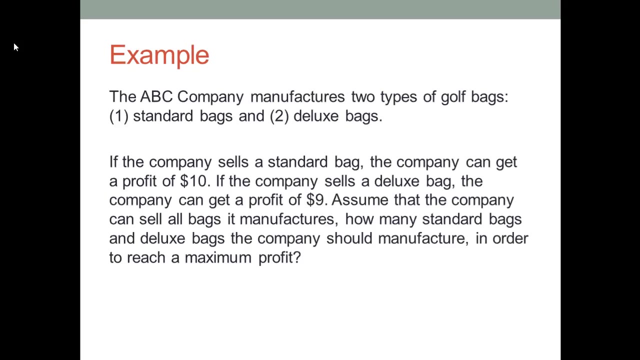 I listed the linear programming fundamental lecture videos link in this video's description section. Please review those videos in order to get familiar to the concepts in linear programming. I will not repeat the fundamentals here. Next I want to use an example to show everyone how to use Python to perform linear programming. 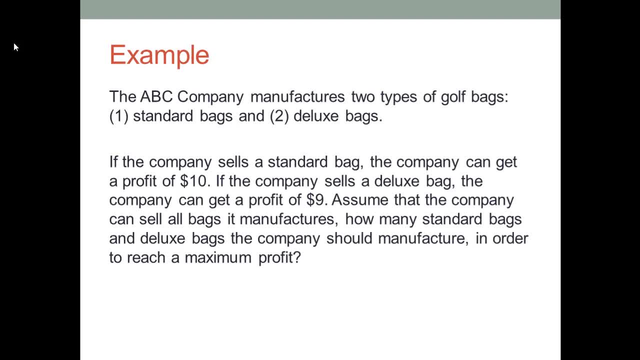 A company wants to maximize the profit by selling two types of bags: standard bags and deluxe bags. If the company sells a standard bag, the company can get a profit of $10 from each standard bag. If the company sells a deluxe bag, the company can get a profit of $9 from each deluxe bag. 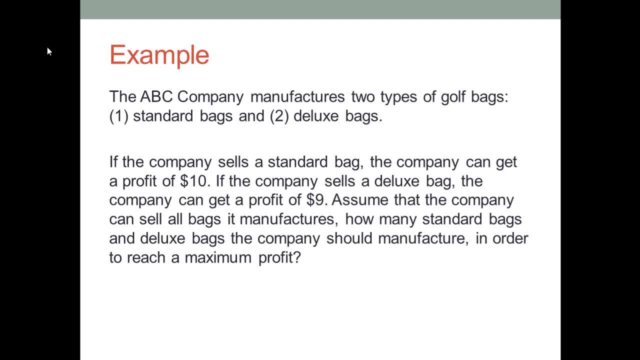 The manager wants you to calculate how many standard bags and deluxe bags companies should sell respectively in order to maximize the total profit. We need to use the guideline we just discussed to identify the objective variable and decision variables. for this case, The objective is to maximize total profit. 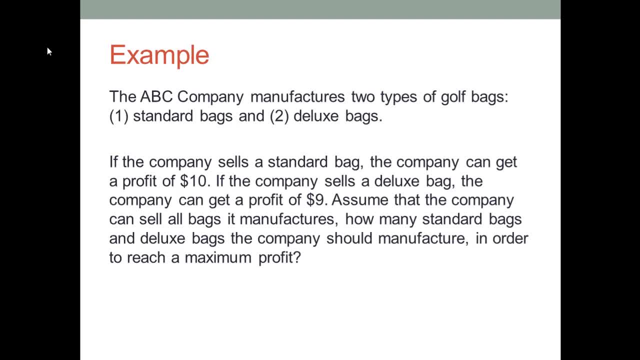 How can we calculate the profit? The total profit is dependent on the number of bags we should sell in each type. Let's use letter S to denote the number of standard bags we will sell in a total, And we use the letter D to denote the number of deluxe bags we will sell in a total. 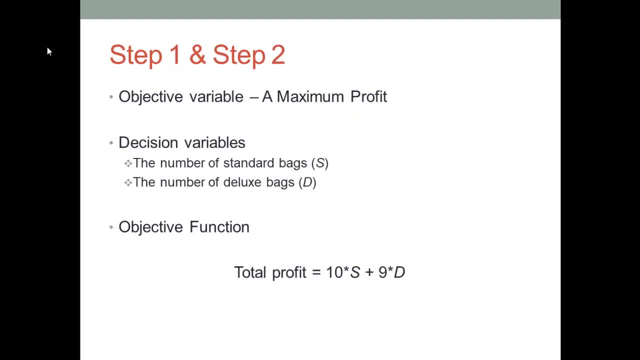 Then we can build an objective function like this one. Total profit equals to 10 times S plus 9 times D. According to this objective function, we can see that the more bags the company sells, the more profit the company will get if the company doesn't have any manufacturing capacity limit. 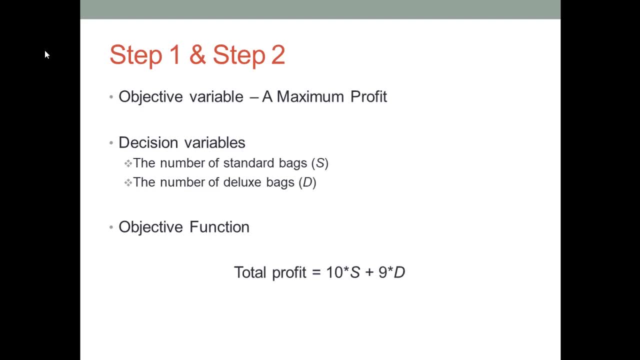 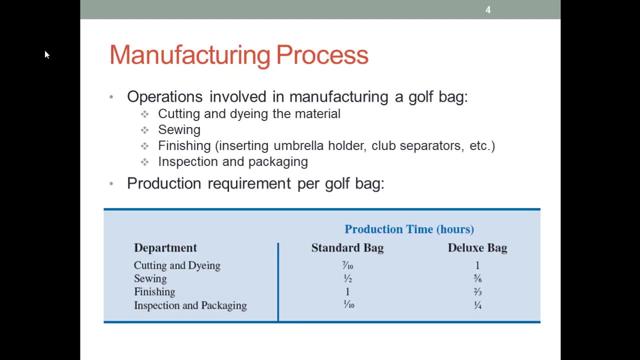 But that's impossible. in reality, The company is facing the manufacturing limit. Let's take a look at those constraints. In order to manufacture one bag, this bag will go through four departments in this company: Cutting and dyeing, shoeing, finishing, inspection and packaging. 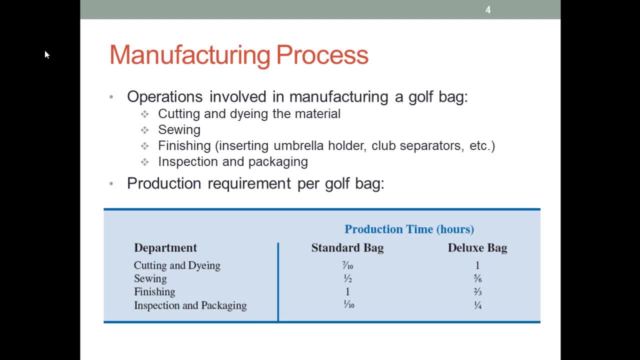 The table on this slide shows everyone how long it will take for one bag to go through one department. Let's use the standard bag as an example. Let's say we want to manufacture a standard bag, Then it will take Cutting and Dyeing department 0.7 hours to manufacture this standard bag. 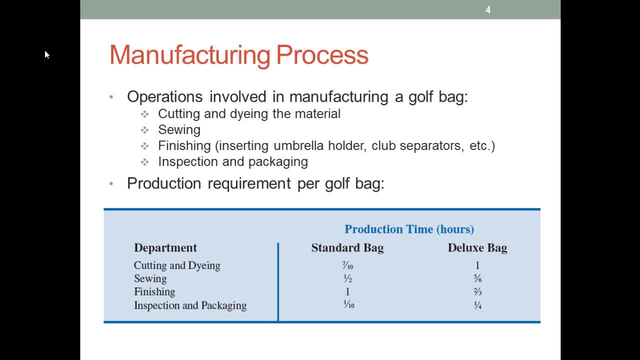 Once this department is done, the bag will move to the next department. According to the table you can see, it will take the Shoeing department about 0.5 hours to manufacture one standard bag. Then the standard bag will move to Finishing department. 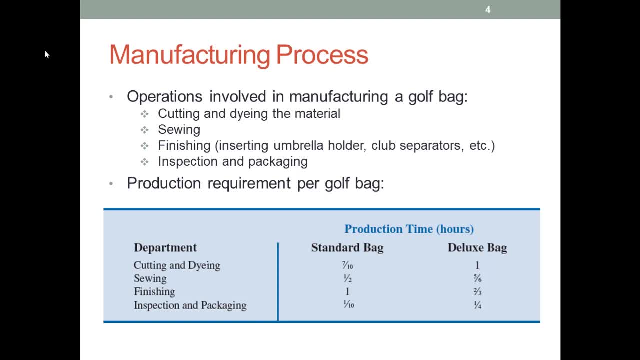 It will take one hour for Finishing department to manufacture this bag. Then it will move to the last department, Inspection and Packaging. It will take about 0.1 hours for this department to finish up this standard bag. Of course, this table also shows everyone how long it will take each department to manufacture a deluxe bag. 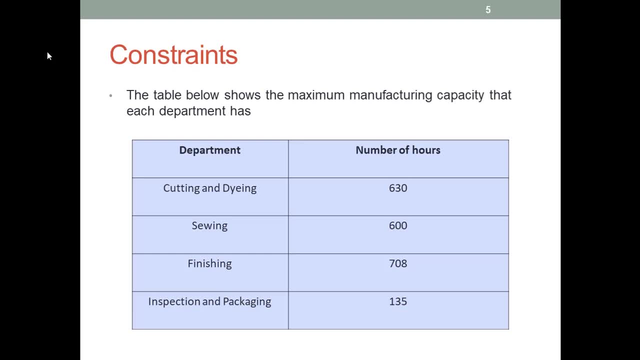 No matter how many standard bags and deluxe bags you want each department to work on, they are all facing capacity limits. For example, the available hours in Cutting and Dyeing is 6.30.. The available labor hours in Shoeing is 600, and so on and so forth. 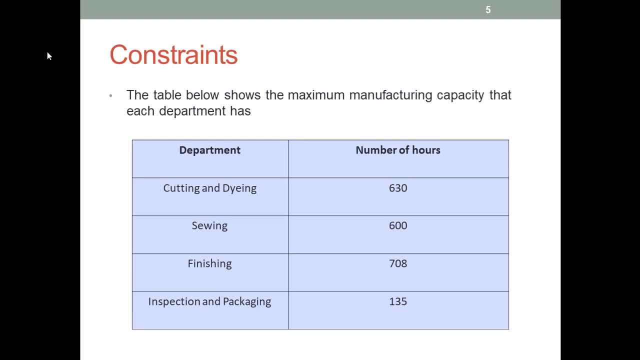 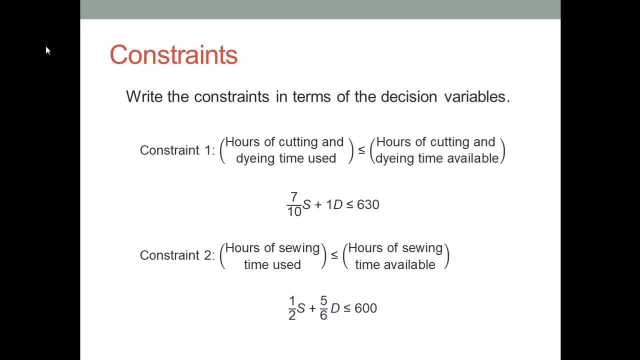 How can we transform these capacity limits into constraints? Here they are. Let me use Cutting and Dyeing as an example. We just said it takes Cutting and Dyeing 0.7 hours to manufacture one standard bag, And we want the company to manufacture S units standard bags. 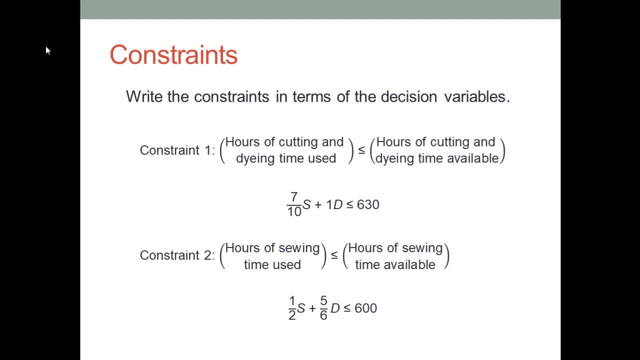 So the total hours we need from the Cutting and Dyeing department for manufacturing total standard bags should be 0.7 times S. We also said it takes Cutting and Dyeing 1 hour to manufacture one deluxe bag. We want the company to manufacture D units. 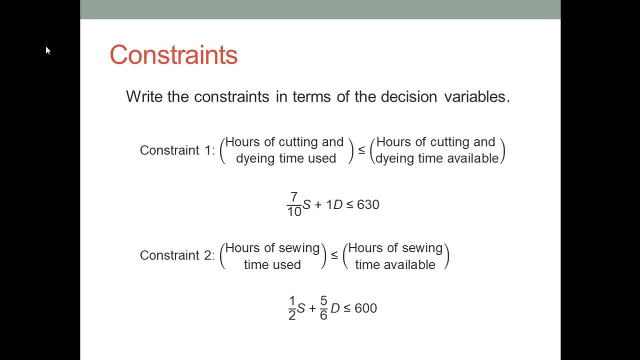 So the total hours we need from Cutting and Dyeing to manufacture D units- deluxe bags- should be 1 times D, 0.7 times S plus 1 times D is the real number we need from the Cutting and Dyeing department. 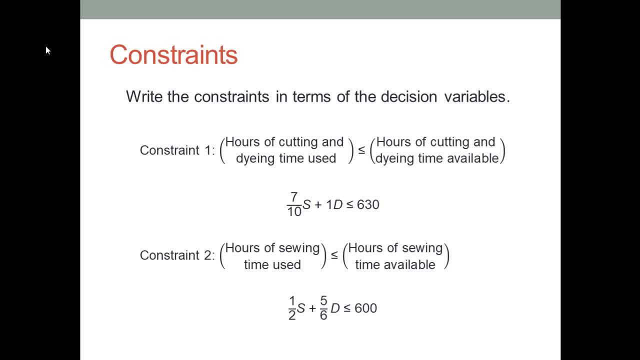 No matter how long it will be. 0.7 times S plus 1 times D cannot exceed the capacity limit of Cutting and Dyeing department. Therefore, 0.7 times S plus 1 times D should be less than or equal to 6.30 hours. 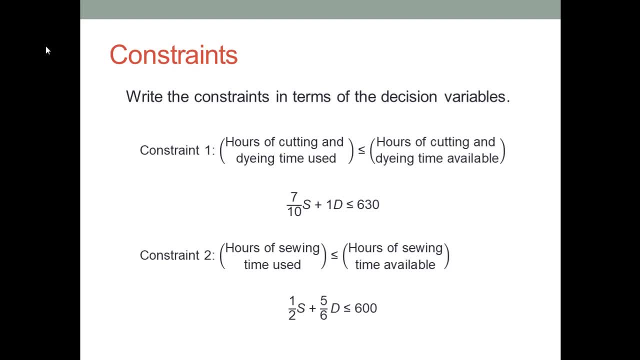 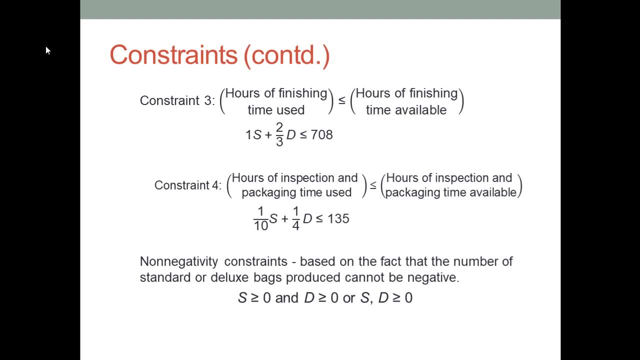 You can use the same logic to build other constraints for other departments, as you can see on this slide and the next slide. I will not repeat it here. Here we also have an implicit constraint: No matter what the value for S and D will be in the future, they cannot be negative. 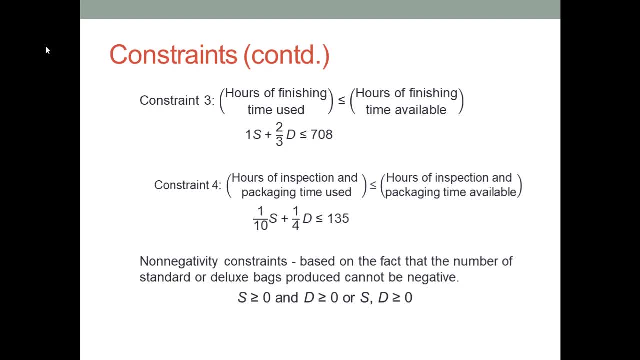 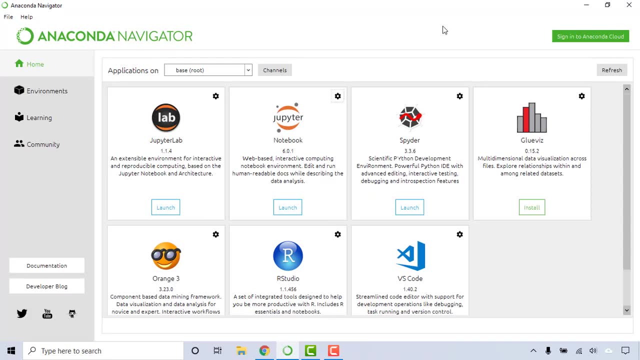 So we have S greater than or equal to 0 and D greater than or equal to 0.. Let's use Python to answer this question. Python is very powerful. However, Python doesn't offer linear programming packages directly. We have to use some third-party packages. 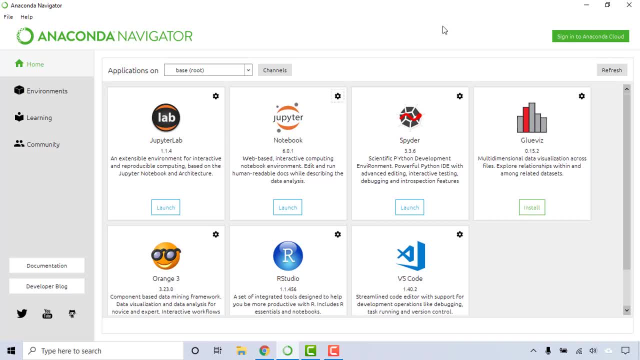 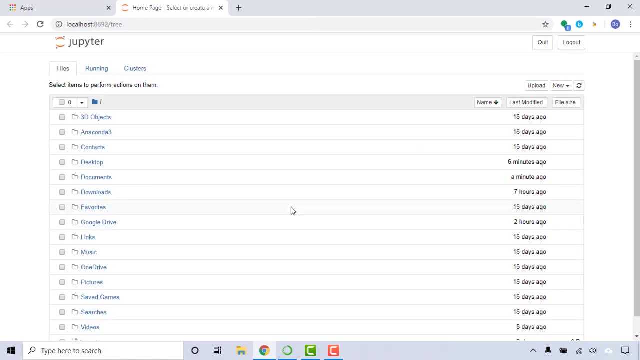 There are tons of options. In this lecture, I want to showcase the PULP function. Let's take a look at it. Let's launch Jupyter Notebook. By the way, if you haven't installed Jupyter Notebook, I listed the installation guide in this video's description section. 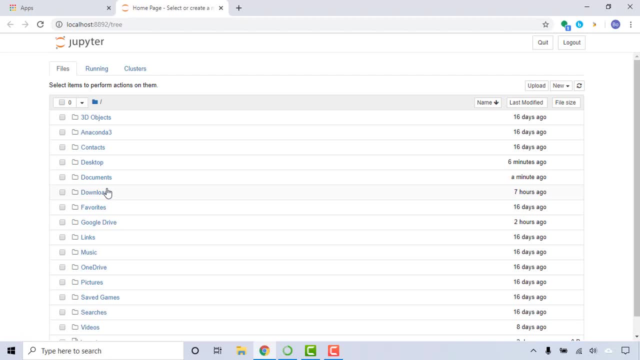 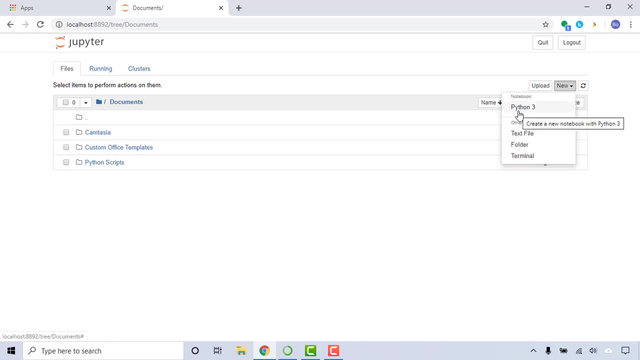 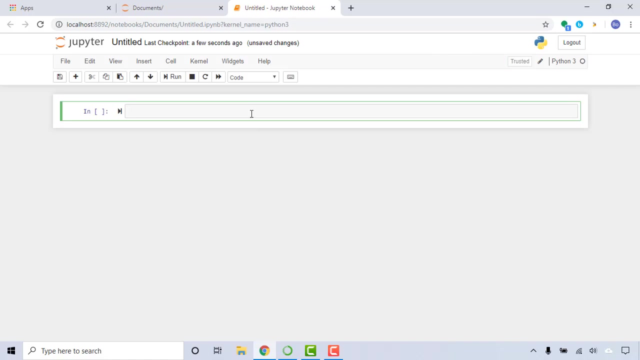 You can find a folder to save the Jupyter Notebook file. I will save it into Documents And then click New in the top right corner And then choose Python 3.. If you haven't installed the PULP function, you need to use the pip function to install it. 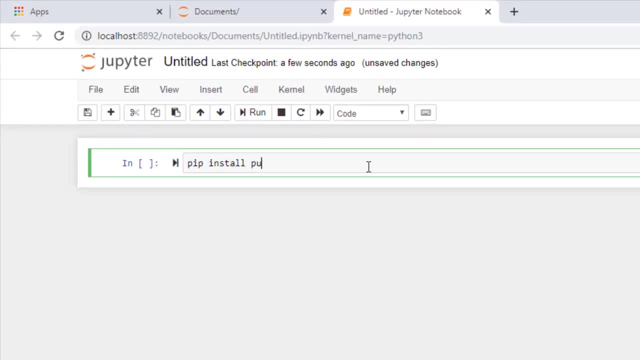 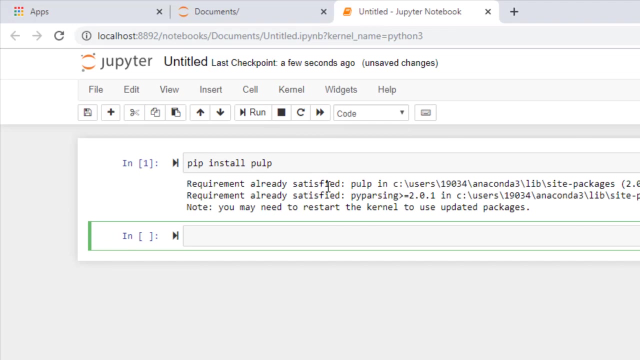 The line is pip- install pulp. pulp is the pop function package name And then click Run. I have installed it So you can see all requirements are satisfied. If you install pop for the first time, you will see a message showing you your installation is finished. 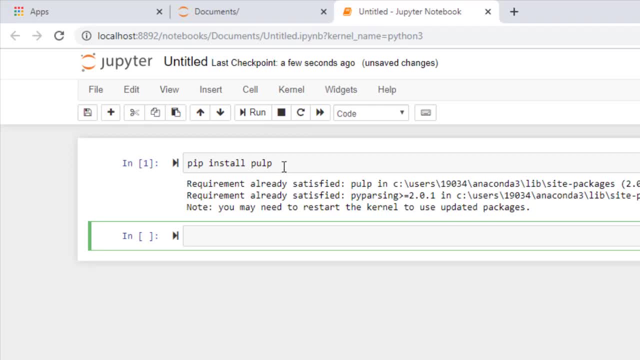 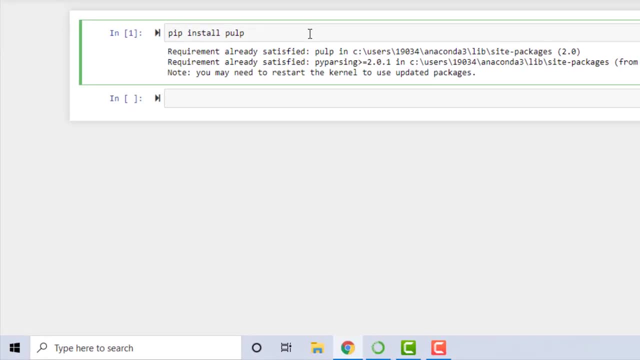 Once the installation is done, you don't have to install it for the next time. You just need to install it once. Now we can use the PULP package. Let's find a new cell in Jupyter Notebook and then type in: import- PULP. 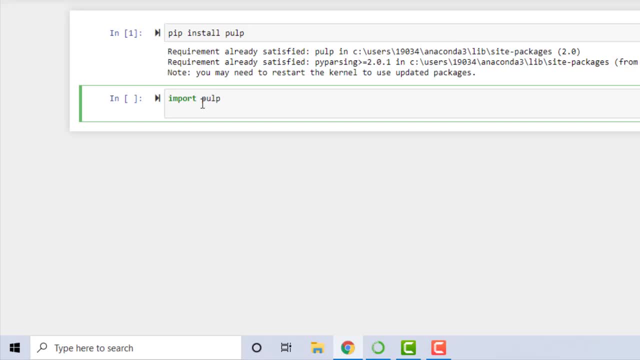 We want to let the Jupyter Notebook know that we want to use the PULP package First. we need to use the LP variable function in the PULP package to define decision variables. I want to use the letter d to denote the number of deluxe bags we want to manufacture. 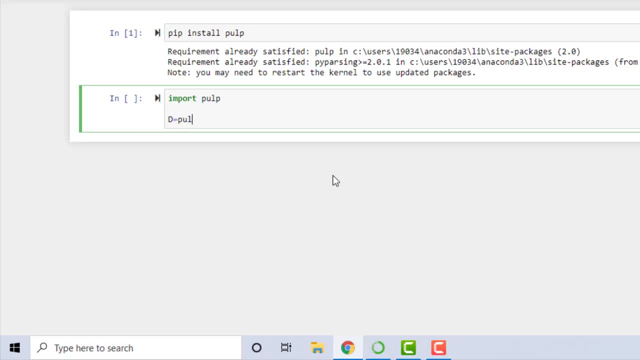 d equals to pulp, dot lp variable. and then parentheses. Between parentheses, we want to type in two single quotes, And then, between two single quotes, we want to type in d. We want to let the PULP package know that letter d is to denote. 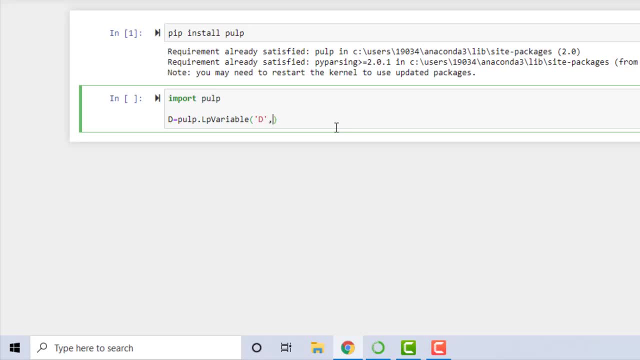 a decision variable And then a comma. After the comma, we want to type in the low bound option. Low bound equals to zero. This means no matter what the value for d is, d cannot be negative. d must be greater than or equal to zero. 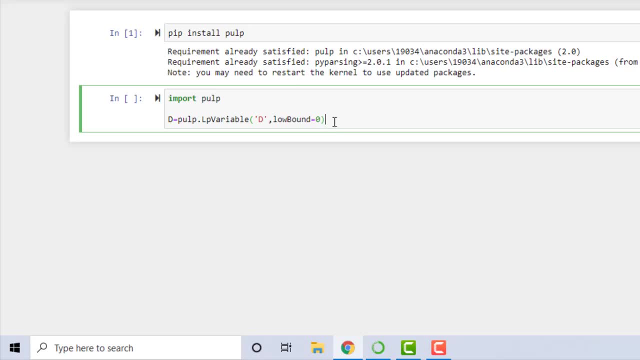 And then I want to use letter s to denote the number of standard bags we want to manufacture. Basically, you can copy the d line and then paste it and then change to s equal to pulp dot. lp variable. Change d to s uppercase s, and the low bound for s is also zero. 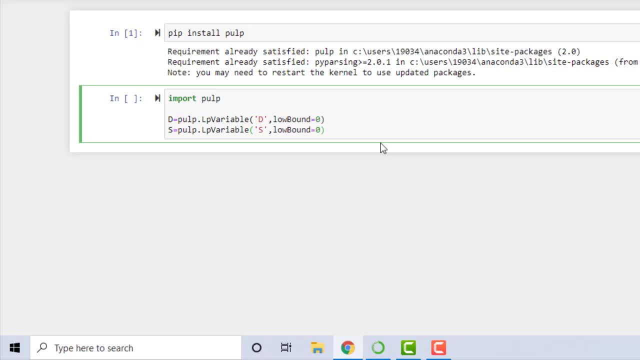 s must be greater than or equal to zero, Non-negative. This is how we define the decision variables in PULP function. Next we need to build the objective function. I want to use the variable profit to represent the objective variable. Let's type it in. 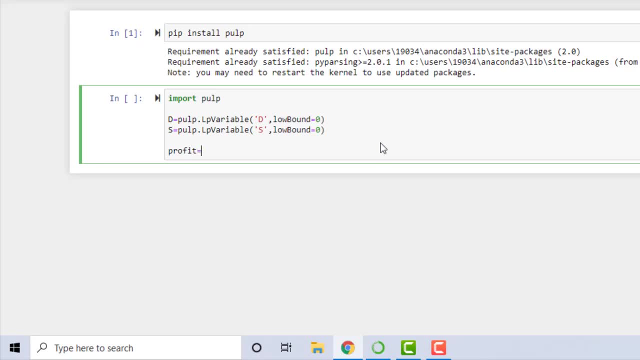 Profit equals to pulp dot lp problem. And then parentheses. Between parentheses, we need to specify two values. First we need to specify a value. Let's type in two single quotes. Between the single quotes, we need to type in maximum profit. 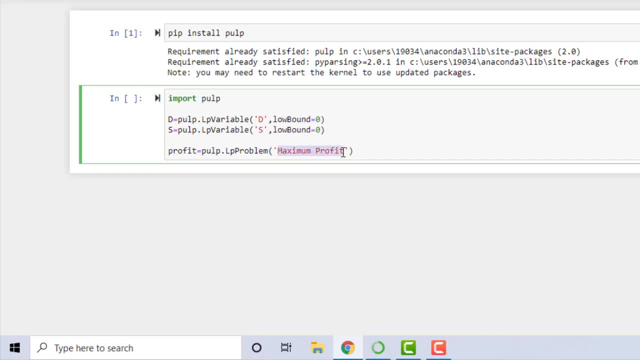 Here, maximum profit is just a label to show the purpose of this analysis, And then a comma, And then we need to type in pulp dot lp maximize. Now we need to let the PULP package know that we want to create a variable profit. 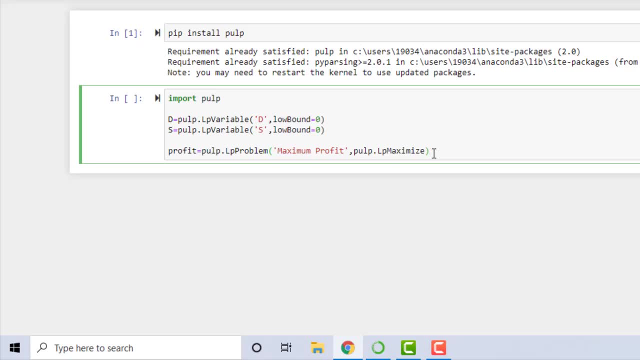 to represent the objective variable And we want to find the maximum value for this objective variable. That's why after the comma we type in pulp, dot lp- maximize. We want to find the maximum value. Next we want to build the objective function. 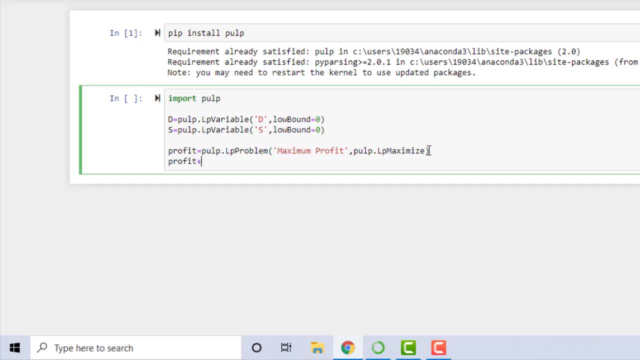 Profit plus equal to 10 times s plus 9 times d. Here you find a new symbol. plus equal to. That means we want to keep adding some functions into the variable profit. You can also add some notation for this function Type in a comma. 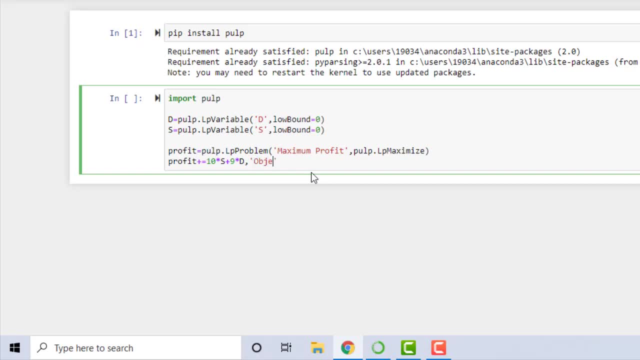 and then two single quotes And then you can see objective function. Notice that the notation is optional. If you don't want to add the notation, you simply remove comma and the notation, You just type in the objective function. But if you want to make the objective function, 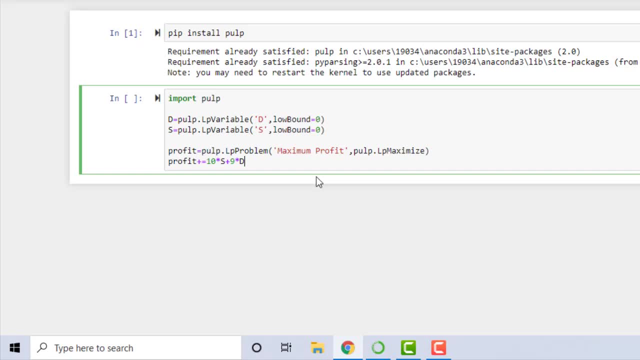 more readable to other data users and programmers. you can add the notation A comma and then includes the objective function. this notation between two single quotes, But it's optional, And then we can add the constraints into profit: Profit plus equal to. 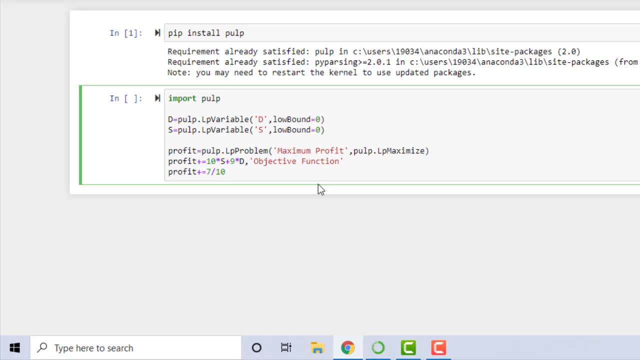 7 divided by 10 times s plus d, And this total must be less than or equal to 630, the capacity limit of the cutting and dying department. You can also add a notation Comma, two single quotes. You can write constraint. 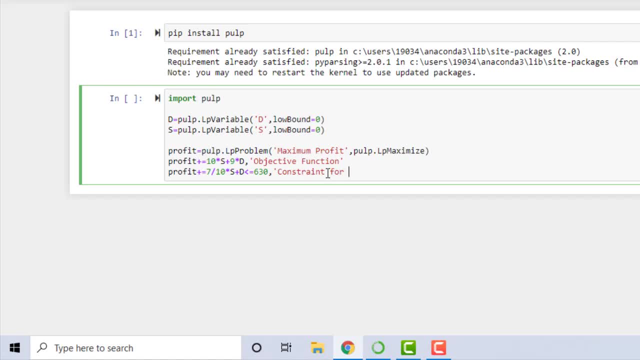 You can add a constraint for cutting and dying And then we can copy this line And then paste them into other constraints. Profit for the second department, showing 1 over 10,, 1 over 2 times s plus 5 over 6 times d. 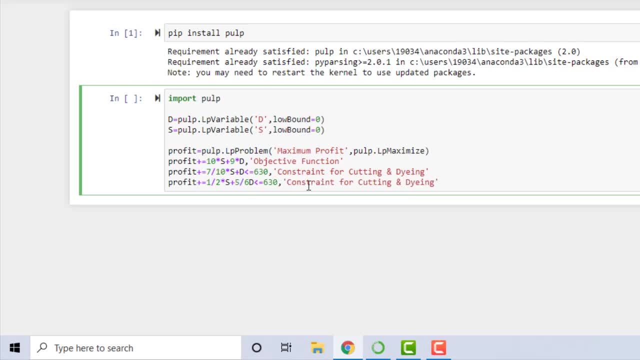 1 over 2 times s plus 5 over 6 times d, Less than or equal to 600.. You can find the constraint requirements in the point points. I listed the point points in this video's description section. This is the constraint for suing. 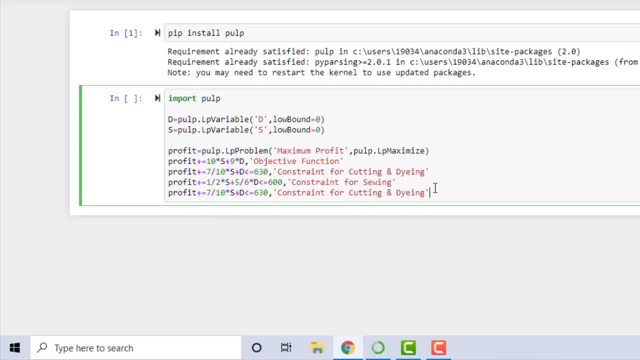 And then you can keep pasting the first line: Profit plus equal to s plus 2 divided by 3 times d, And this total must be less than or equal to 708.. And this is the constraint for finishing department. And then the last constraint is: 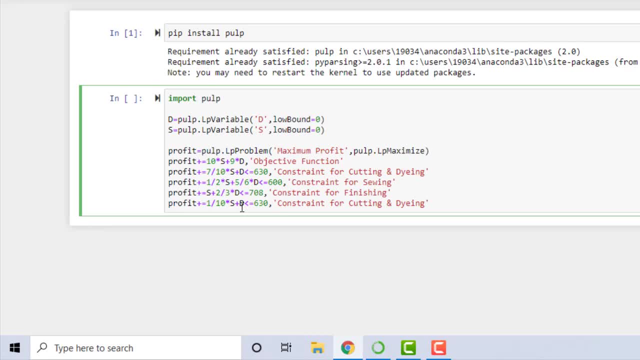 1 over 10.. 10 times s plus 1, divided by 4 times d, This total must be less than or equal to 135.. This is the constraint for inspection and packaging department. I will use imp to represent this. Then we are ready to solve this question. 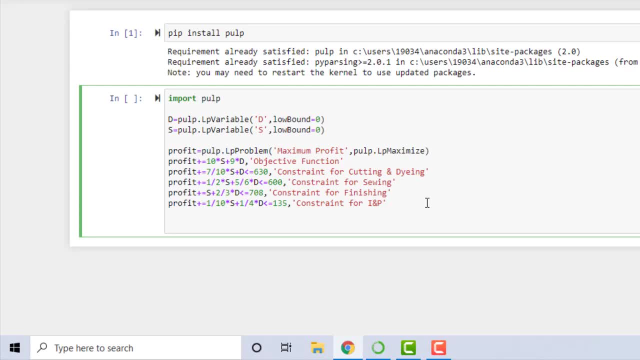 The function of solving a linear programming question is solve function. You just type in profit dot solve. Basically this means you give every objective function constraint into the variable profit, So the profit has the linear programming system And then you use the solve function to find the value. 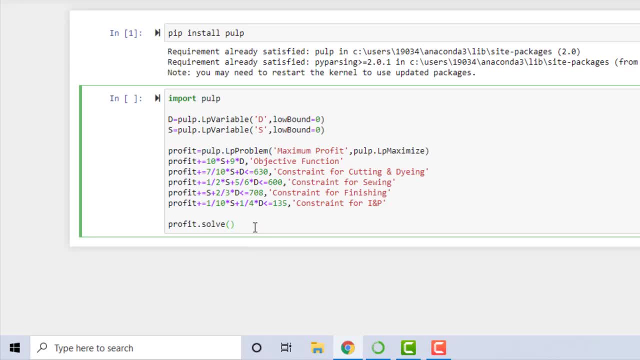 If you want to see the results right First. you want to see the values for decision variables. You want to figure out how many standard bags and deluxe bags we want to manufacture. Then you can use the for loop to find the values. 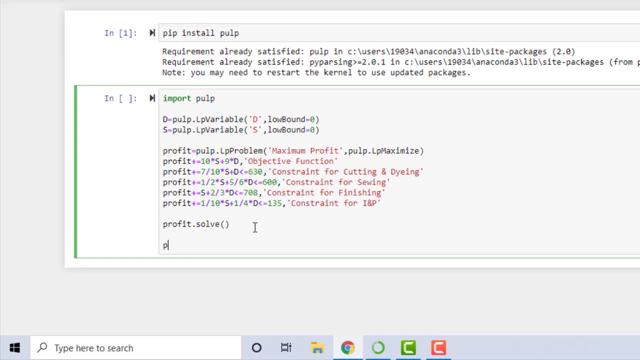 Let me type it in. First let's add a label, Let's type in print decision: variable values And then, after the print function, let's use a for loop to find the value For variable in profit dot variables. Print- Print. 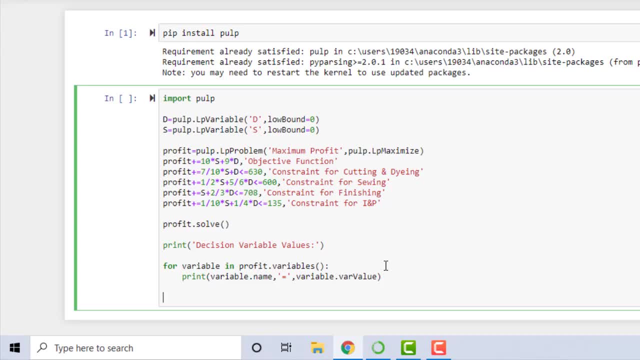 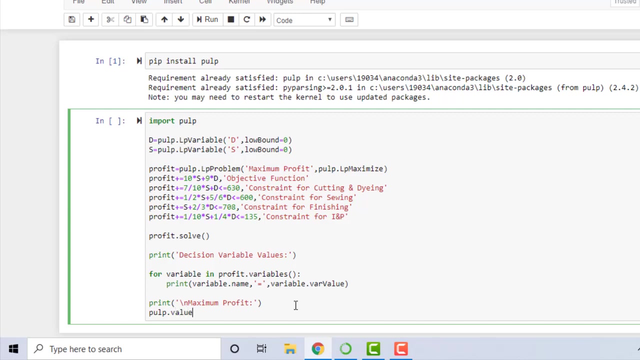 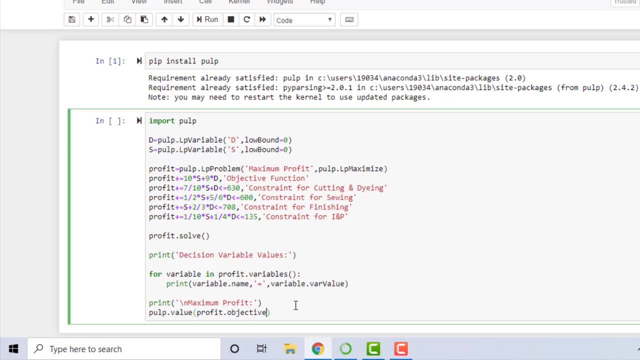 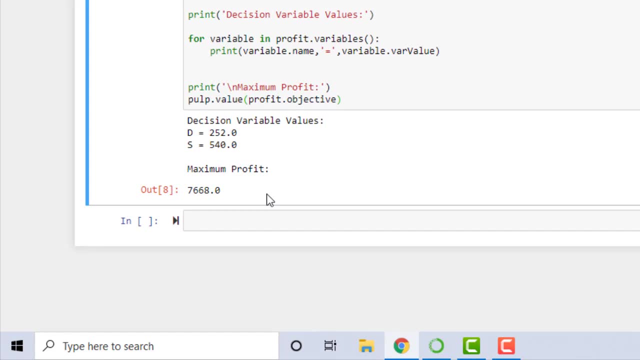